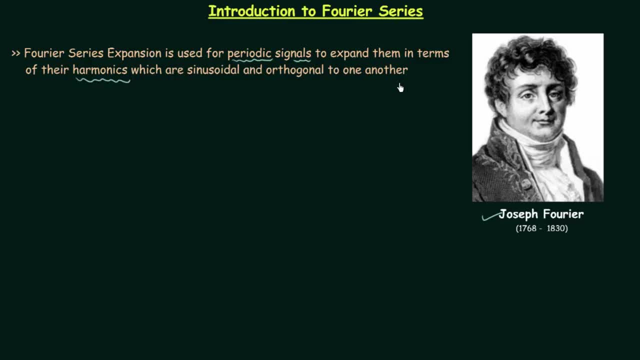 These signals are синusoidal and orthogonal to one another. We will try to understand the meaning of this statement. The first important thing which we can seek is the use of Fourier series expansion only incase of periodic signals. We already know what are periodic signals. 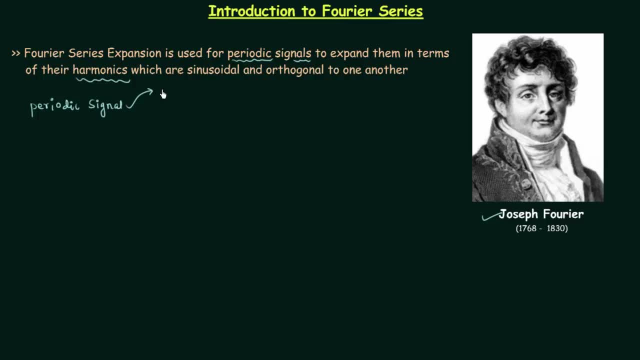 There are 2 Types of periodic signals. The first one is continuous time periodic signals and the second one is discrete time periodic signals. Now, based on continuous time and discrete time, we have two types of Fourier series expansions. For continuous time, the Fourier series expansion is known as continuous time Fourier series. 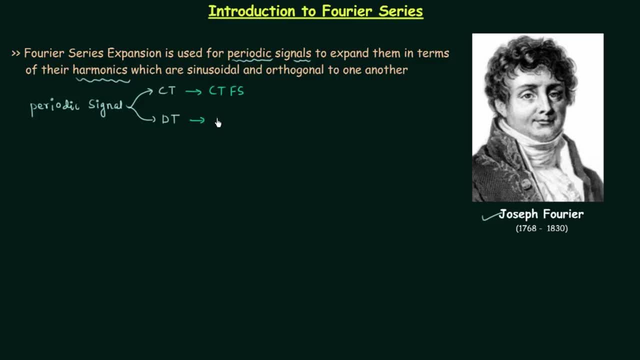 and for discrete time, the series is known as discrete time Fourier series. In this particular chapter we will only discuss continuous time Fourier series expansion and once we complete discrete time signals, we will move on to discrete time Fourier series expansion. Now we have the Fourier series expansion. 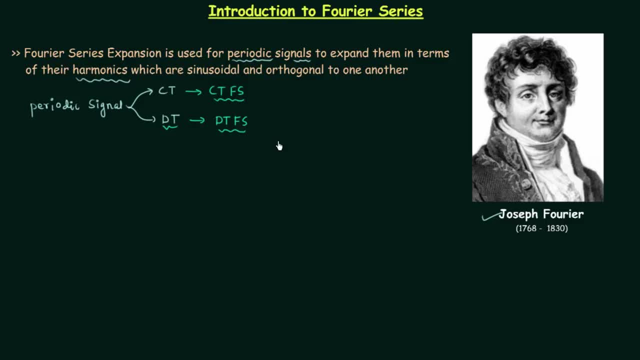 Now, what is the use of obtained expansion? We use Fourier series expansion for the analysis of the Fourier series. What is its purpose? And now you will ask, when we have Fourier series, then why we moved on to Fourier transform? To understand this, you have to focus on the first important point mentioned in the above. 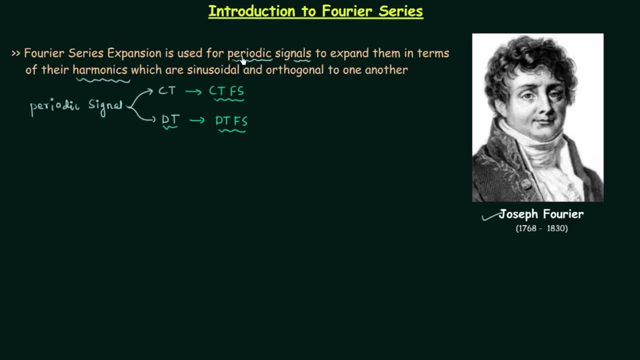 statement: Fourier series expansion is used for periodic signals only. Now, what about non-periodic signals? This is for periodic signals. What about non-periodic signals? If we talk about real life signals, Then we don't have the periodic signals. Generally, we have the non-periodic signals. 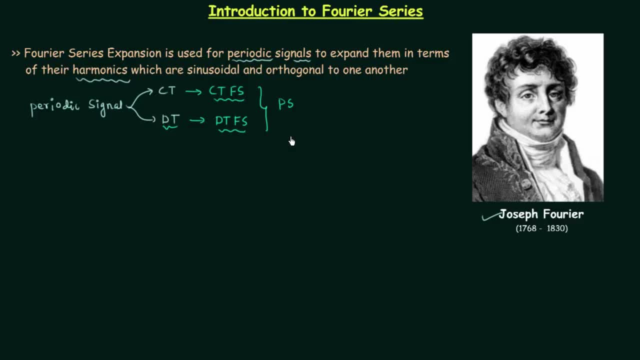 We will see one example of this after few minutes. But we know the real life signals are non-periodic in nature. Now, for analysis of non-periodic signals, we needed some tool, And the tool was given by Joseph Fourier, and the tool is known as Fourier transform. 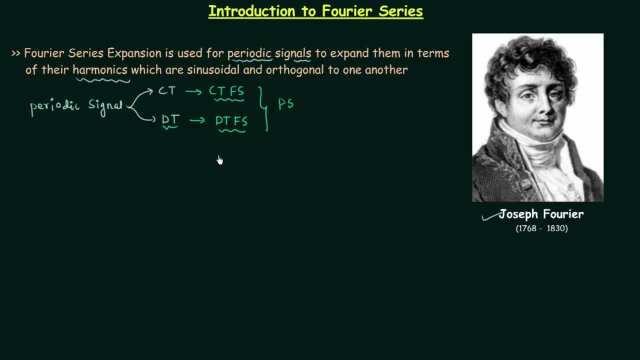 Now there are two types of non-periodic signals. The first one is continuous time, The second one is continuous time. The third one is continuous time- non-periodic signals, And for this we have the tool known as continuous time Fourier transform. In the same way we have discrete time Fourier transform. 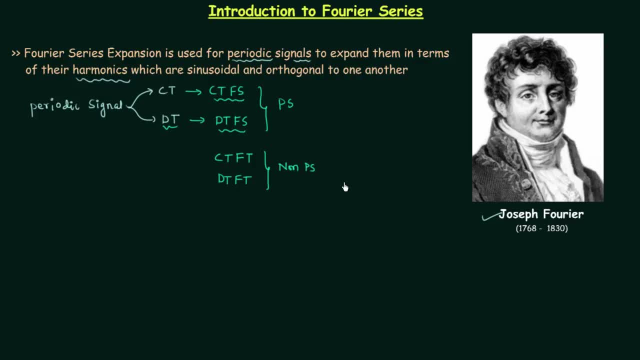 And they are for non-periodic signals. So I hope you now understand what is the difference between Fourier series and Fourier transform And why we have continuous time Fourier series, Discrete time Fourier series, Continuous time- Fourier series. But again, you will ask me what is the use of Laplace transform? 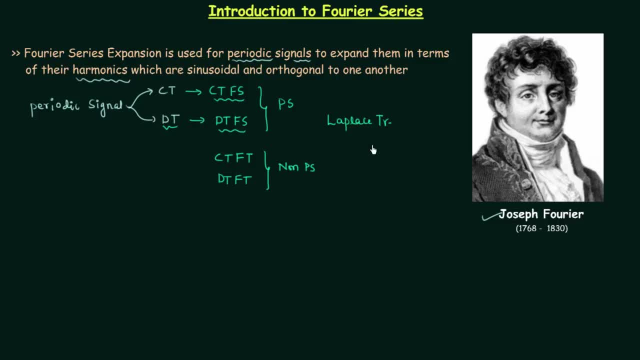 Laplace transform is used for designing. Fourier series and Fourier transform are used for e快 transition. Fourier series and Fourier transform are used for analysis purposes, where as Laplace transform is used for designing. So you can вы not get confused. 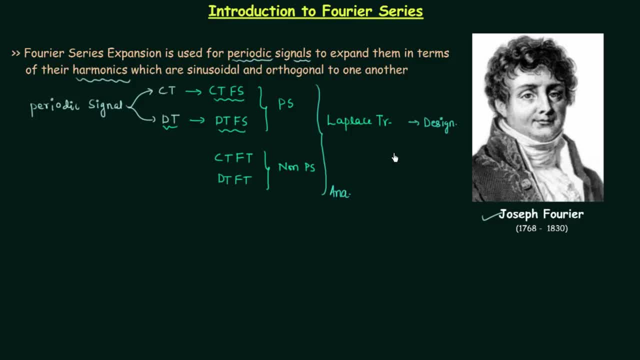 designing purpose. We obtain the transfer function using the Laplace transform and by using the different methods available, we can easily check the stability of the system and, by using the results obtained, we can design our system. Now you will ask me: what is Z transform or Z transform? Laplace transform is for continuous time and Z transform is for discrete time. So I hope you now understand the difference between Laplace transform and Z transform, and they are all important chapters of this particular course. 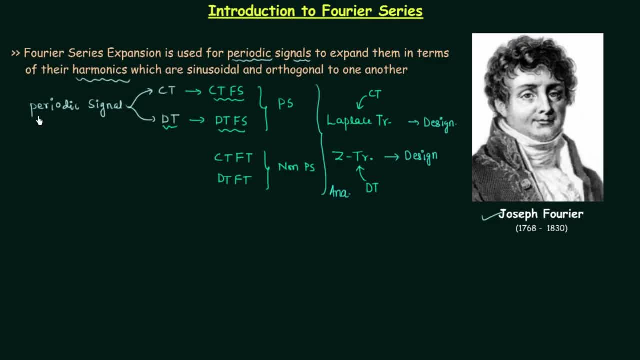 Now we will move back to our discussion. We have all already completed Periodic Signals. If you have not seen the lectures on Periodic Signals, you may watch the lectures by following the playlist. There I have explained every important point related to Periodic Signals. 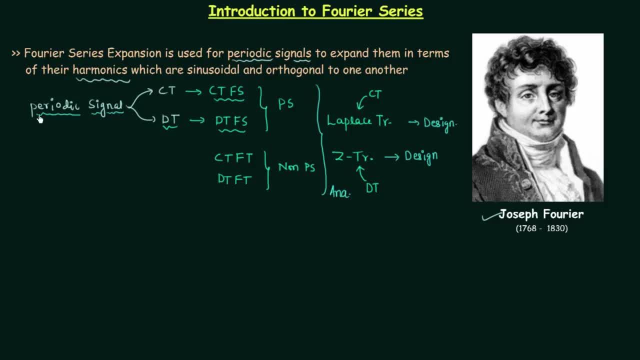 We have also solved various numerical problems based on Periodic Signals. But for the explanation purpose I will quickly explain what do we mean by Periodic Signals. Periodic Signals are those signals in which there is repetition of a particular structure from minus infinity to infinity. Or you can say: Periodic Signal is a signal in which the signal repeats itself after a particular interval of time. 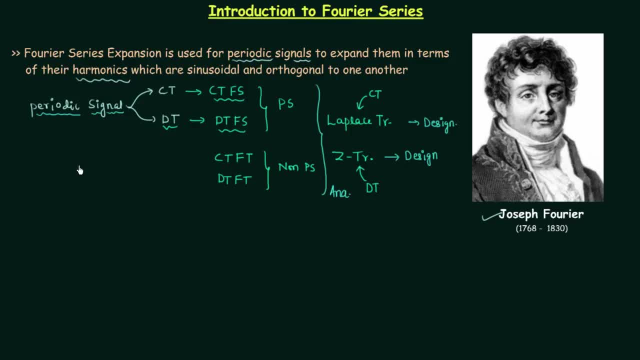 And this particular interval of time is known as Time Period of this signal. So if we have a Periodic Signal- X, that is a Periodic Signal- Then we can say that Xt plus minus t is equal to Xt. This is the condition for a signal to be periodic. Now let's try to understand the meaning of this. It says t is a time period. It is a time period and it is equal to n times the fundamental time period. 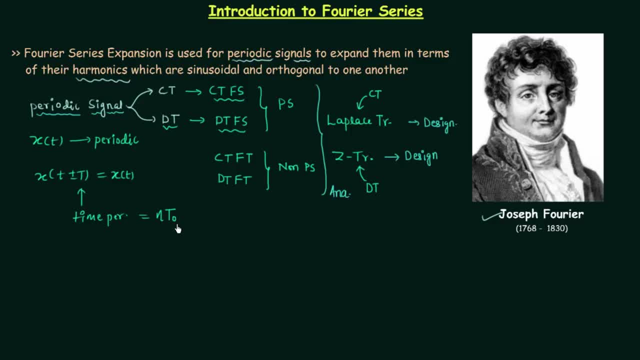 The fundamental time period t0 is the smallest time interval for which the given signal is periodic. And here we are performing the time shifting. We can perform either the left shift or the right shift, but the shifting interval should be the time period. So whenever we perform the shifting towards the left or towards the right by the time period of the signal, we will get the same signal. And we are getting the same signal because I already 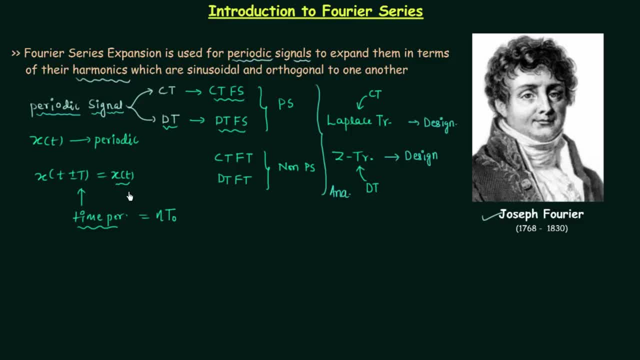 said, the signal is having a particular structure repeating itself from minus infinity to infinity. This point is very important. If the repetition is not from minus infinity to infinity, this condition will not hold true, And if the repetition is from minus infinity to infinity, small shifting will not affect the whole signal. So I hope you now understand, or you now remember what we have already discussed in case of periodic. 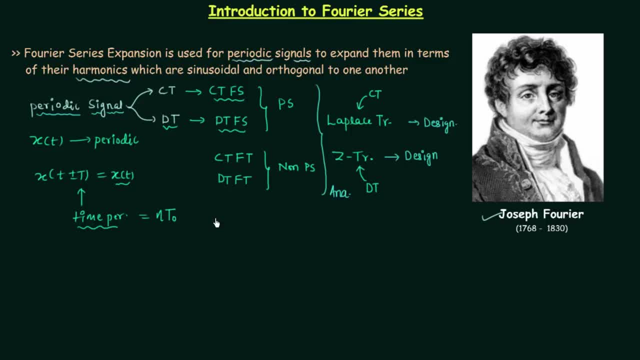 signal. Now we will move to the next important point, And the point is existence of Fourier series. In the statement it is written that Fourier series expansion is used for periodic signals, But it does not mean whenever we have periodic signal the Fourier series expansion will exist. The existence of Fourier series expansion depends on three conditions, and the conditions are known as: 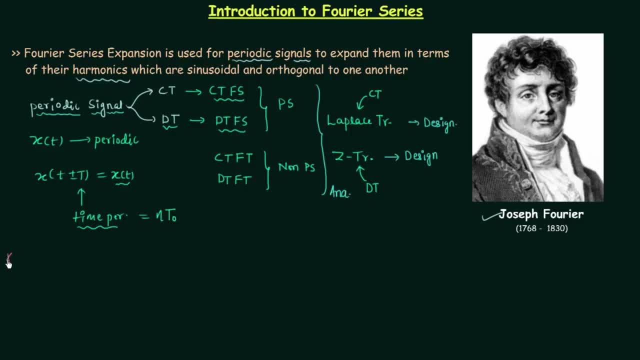 Dirichlet conditions. The conditions are known as Dirichlet conditions. We will discuss Dirichlet conditions in the next lecture. There are three conditions for the existence of Fourier series: expansion: Even if the signal is periodic, the three conditions must be satisfied. 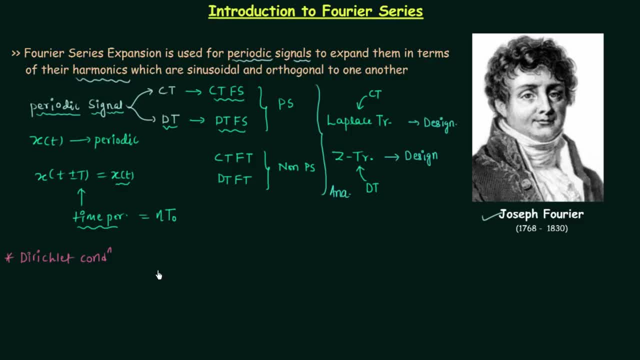 In case of non periodic signals We can straight away say the Fourier series expansion will not exist, exist. but in case of periodic signals we have to focus on Dirichlet conditions and the next lecture is going to be based on the Dirichlet conditions. now we will read the statement further. 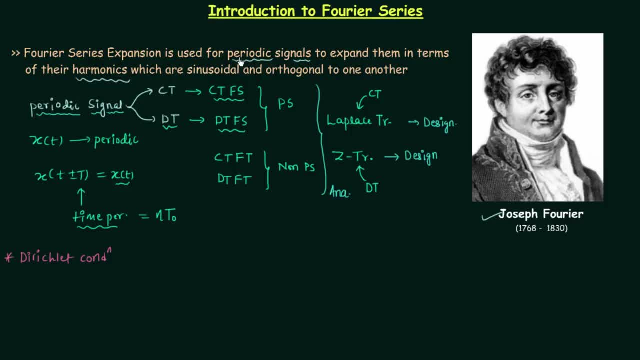 it says the Fourier series expansion is used for periodic signals to expand them in terms of their harmonics. now we have a new term, harmonic, and to understand the harmonic you should understand the frequency first. we know the basic definition of frequency. frequency is defined as the number of cycles per second. it is number of cycles per second and we can easily calculate the. 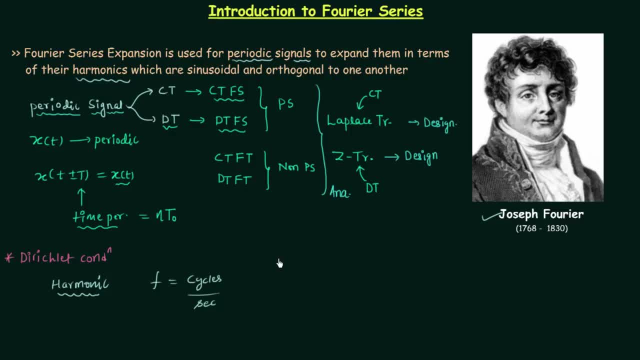 frequency if we have two cycles per second and we can easily calculate the frequency if we have the waveform. I will quickly plot a sinusoidal waveform and I hope you understand what do we mean by sinusoidal waveform. either we can have sine waveform or cosine waveform. here I have 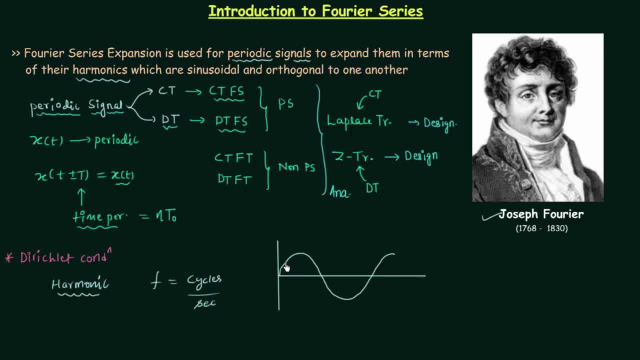 taken the waveform of sine function and you can see one cycle. this is the one cycle is completed from 0 to t. 0 to t is the interval after which the signal repeats itself. so this T here is the fundamental time period, fundamental time period of the sine function, and we can easily calculate. 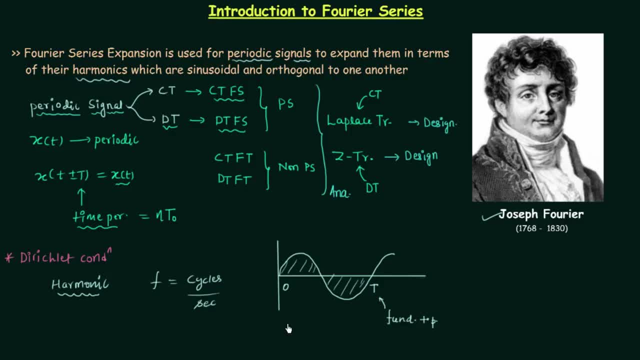 the frequency. it is equal to number of cycles per second. the signal is taking T seconds for 1 cycle. So in one seconds, in one seconds, we will have one over T cycles. Therefore, the frequency is going to be one over T cycles per second, or simply hertz. So this is the definition of frequency and we already know this. But I told you, real life signals are not periodic in nature. For example, I'm speaking right now and my voice is 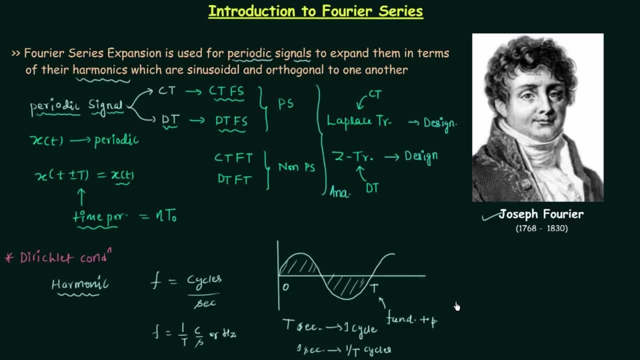 converted to the electrical signal by the help of the mic I'm using. So the mic is having the transducer which is converting my voice to the electrical signal and definitely the signal will not look like this. It is not a periodic signal. It depends on the word I'm speaking and, based on different words, we have different spikes in the waveform, For example, the. 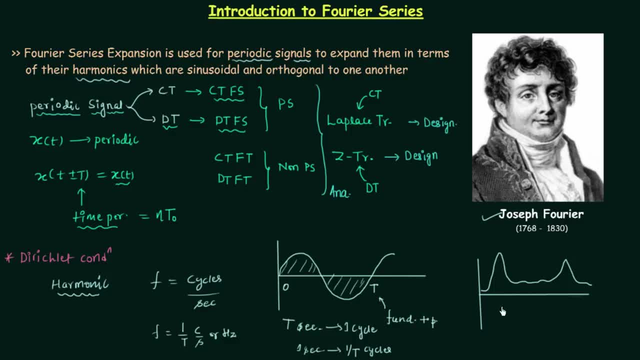 frequency of the frequency signal will look like this forces me to zoom out. Now. you cannot use this formula to calculate the frequency in this case, because you cannot find out the cycles here. Therefore, we need to define the frequency in more general way. The frequency is defined as the rate of change. 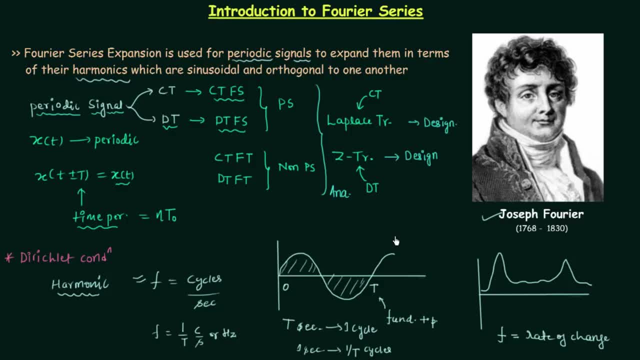 So in this waveform, for example, When I say, say letter C, You can see the variation is not very sharp. I say C. So this portion here in the waveform is when I say letter C And when I say letter T, you can see the variation. 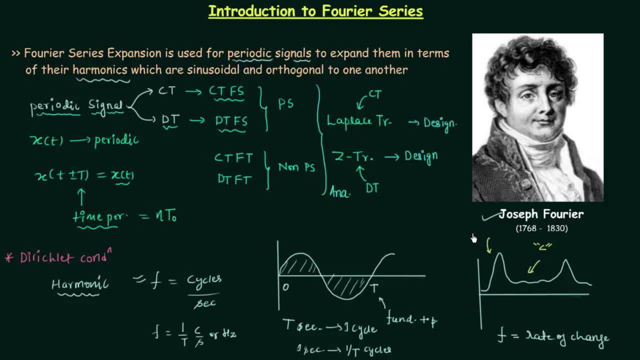 is very sharp. T, So this portion of the waveform is when I say T. So here the rate of change is very high. So this is having the high frequency. Here the rate of change is not very high, So we have the low frequency. In this case we had only one frequency, But here we have. 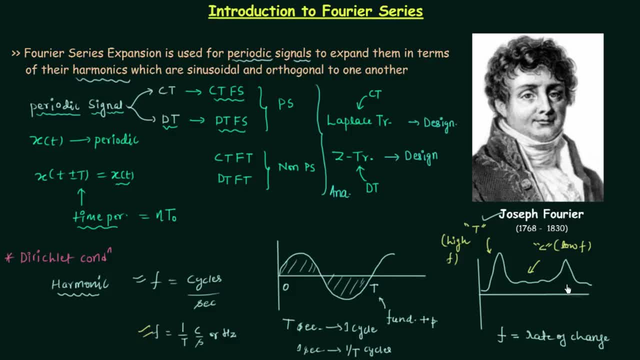 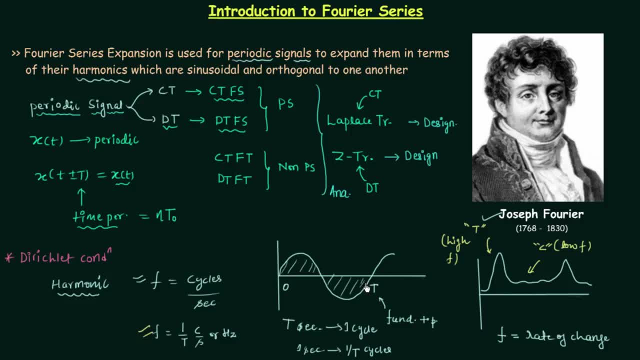 But what do we mean by signal? is that it carries some information? We can say that it is carrying some information because it is carrying something which we don't know. It is non-deterministic, It is random, But here we already know everything about the sinusoidal waveform, either cosine, 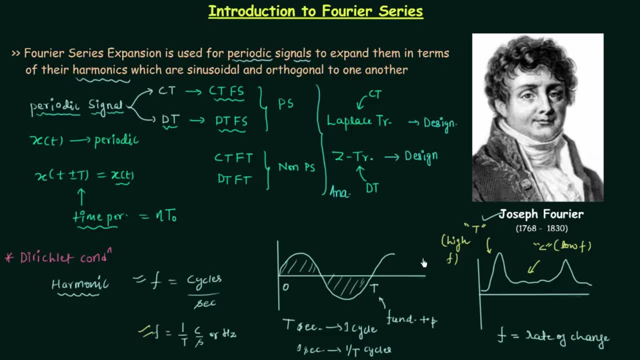 or sine, So it is not carrying some information. Therefore it is practically not a signal. Signal should carry some information And information should not be known to us earlier. So here we have a signal, practical signal, in which there are multiple frequencies available And when we have multiple frequencies, 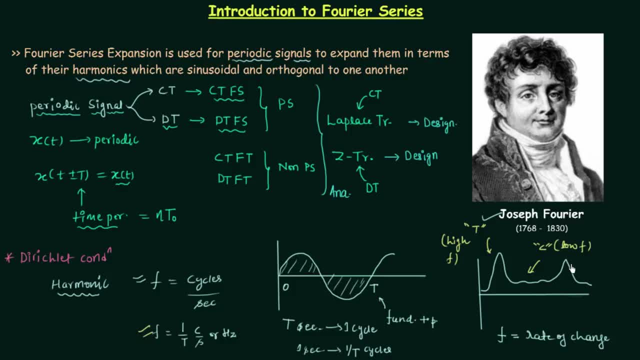 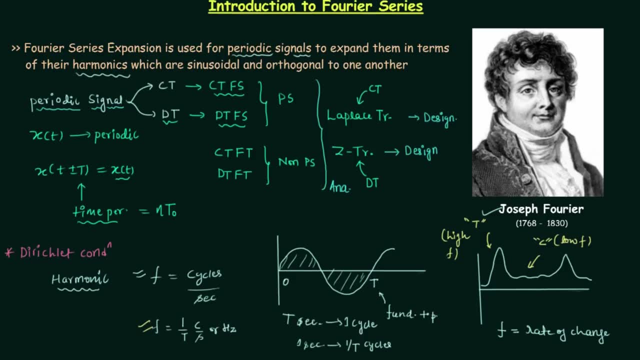 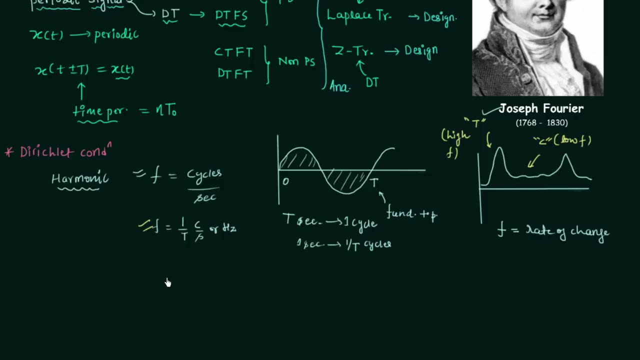 We can have the signal expressed in terms of fundamental component plus the harmonics. Now we will understand what are harmonics. We now know the meaning of frequency And now we will understand the meaning of harmonics. For this I will take one example. In this example, signal Xt is a periodic signal and it is expressed 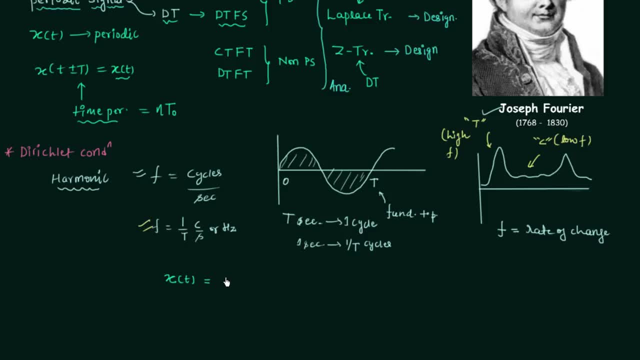 as the sum of original signal and the harmonics. It is equal to twice of sine omega t plus sine two omega t plus seven sine three omega t plus other harmonics. So signal Xt is a periodic signal and it is expressed as sum of original signal and the harmonics. Two sine omega t is. 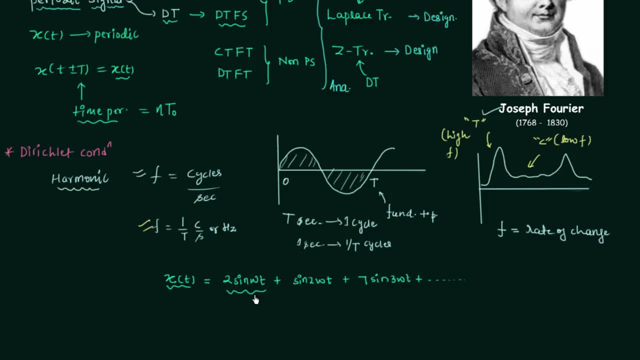 the original signal and it is also known as the first harmonic, because you can see the frequency. here The fundamental frequency is omega. Omega is the fundamental frequency, or more specifically, it is fundamental angular frequency. Angular frequency is equal to two pi f and compared to this, if you see the second term, you will find the frequency is twice of omega. So here the 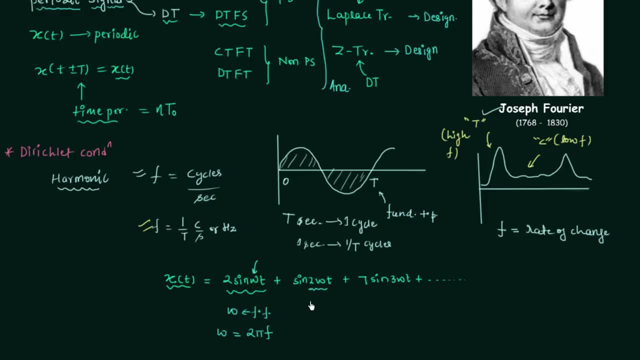 frequency is integral multiple of the fundamental frequency. So whenever you have the frequency as integral multiple of the fundamental frequency, we call the term harmonics. They are not desired in the system generally but they are present In the same way. if you see the third term, you will find 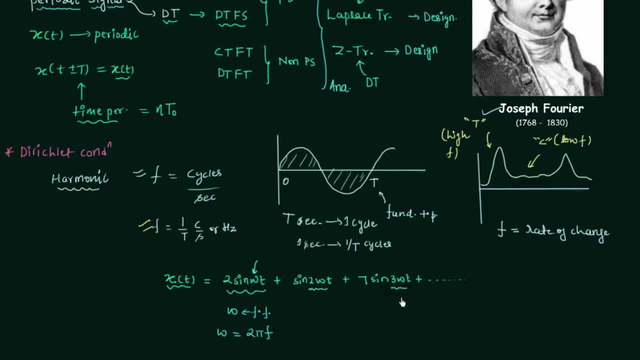 the frequency is three times omega. So again, the frequency is integral, multiple of the fundamental frequency. So this one here is also the harmonic. In the same way we have other harmonics present in this signal and, depending on the integer, here We have even and odd harmonics. Here you can see two omega is there, Two is even. therefore this: 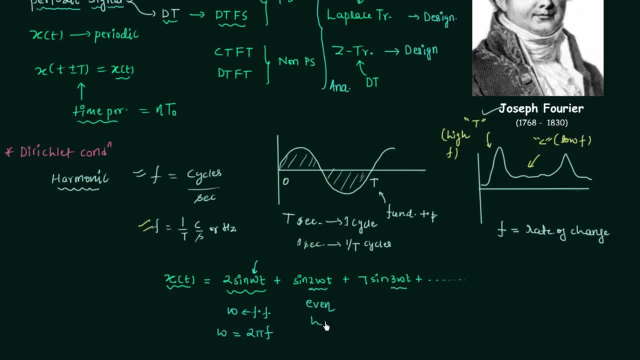 particular harmonic is even harmonic. Here, three omega is there, Three is an odd number. therefore this harmonic is odd harmonic. Now, if you focus on the coefficient, you will find here the coefficient is one, but here the coefficient is seven. Seven is greater than one. So we can say that 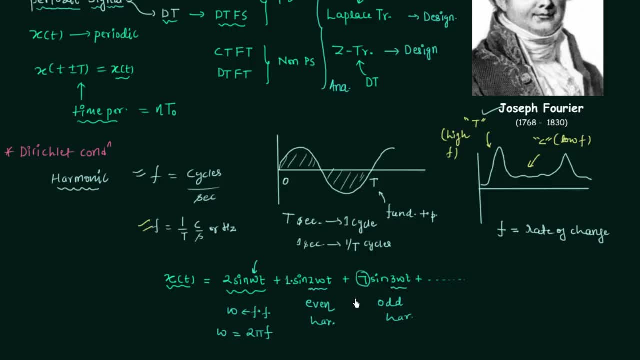 the effect of third harmonic is more as compared to the effect of second harmonic And if the same pattern is followed for the other harmonics also, we can see that odd harmonics are more dominant in this signal and even harmonics are less dominant. It depends on signal to signal. In some 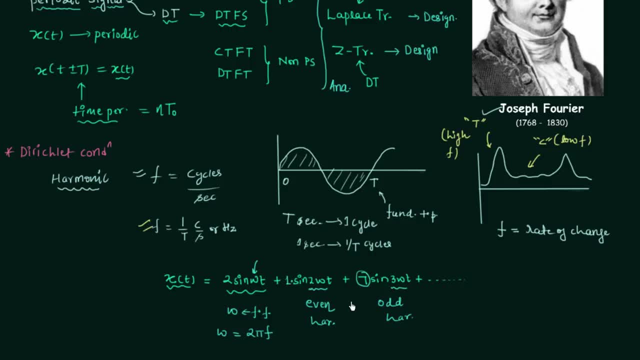 signals, odd harmonics are more dominant. In some signals even harmonics are more dominant and in some signals the dominant signal is more dominant. depend on the integer here. if the integer is larger, the dominance is smaller, and vice versa. so this is all you should know about the harmonic. 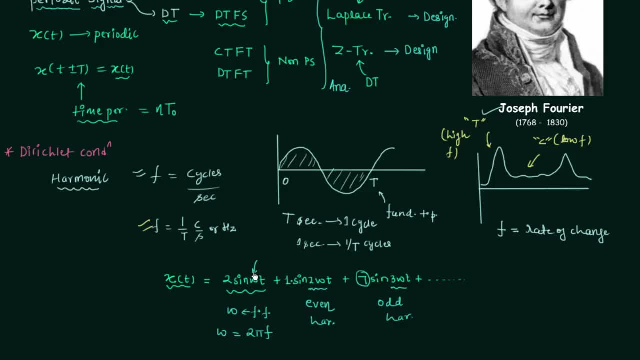 whenever you have different frequency components, along with the fundamental frequency component, we say harmonics are present in the signal. and this is what we want to perform: the analysis. and we can have the same result from the waveform of the signal using the Fourier series. so we want to analyze this signal. 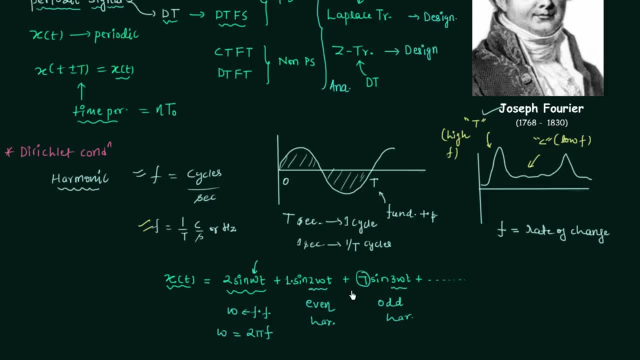 and for that we want to analyze the harmonics present. for example, here we got the information that the third harmonic is more dominant as compared to the second harmonic. so we want this form or this expansion of this signal and we can use the Fourier series expansion for the same. but Fourier series expansion is. 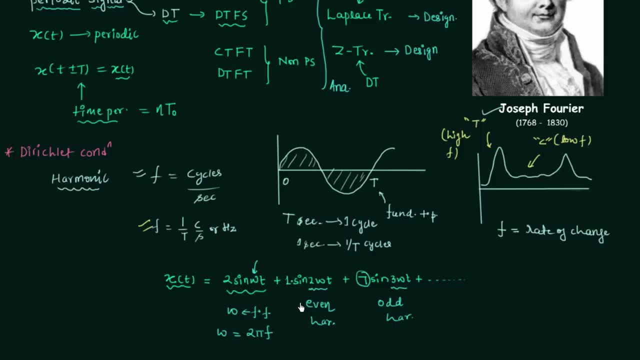 only for this: the periodic signals. so in this chapter we will only deal with periodic signals, and when we have non periodic signals like this, we will use the Fourier transform. by using the Fourier transform we can easily obtain the response known as the frequency response, represented by H Omega. it is complex in nature, so it is. 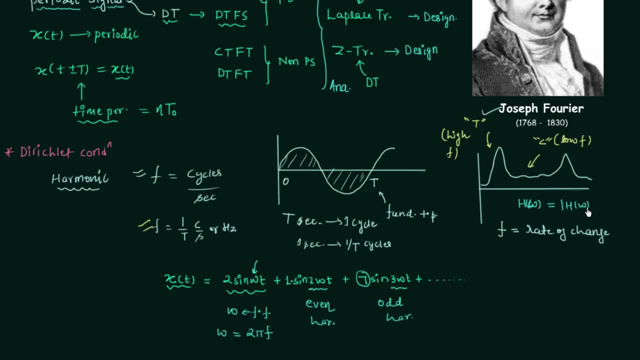 having two parts. the first one is the magnitude, known as the magnitude response, and the second one is the phase of the response, known as phase response. we will talk more about Fourier transform in the next chapter, but for now we will focus on the Fourier series, and we now know why we 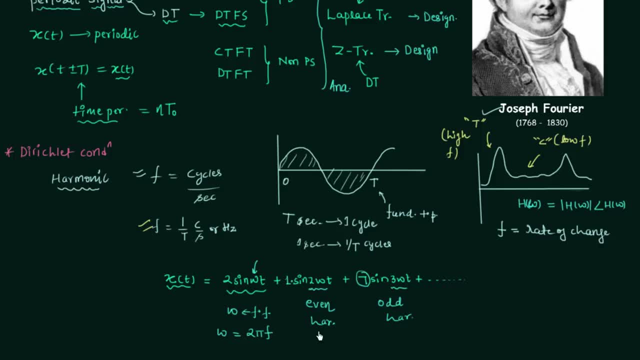 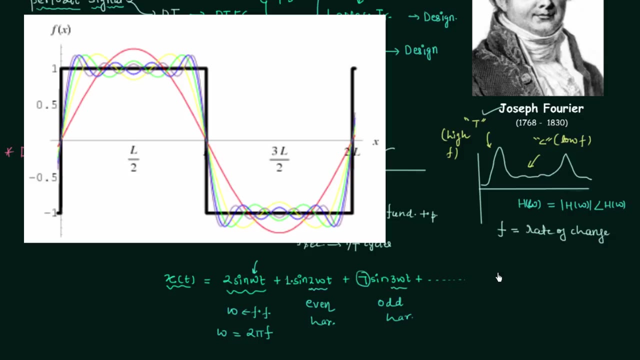 need to obtain the Fourier series. we want this form to analyze the signal and we can obtain this form from the waveform using the Fourier series. now I will show you one example. on your screen you can see the square waveform and in the square waveform you can see different harmonics present. there is fundamental signal and if you try to visualize, 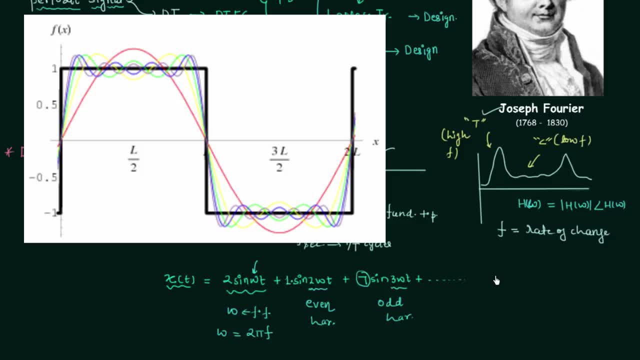 the waveform from minus infinity to infinity, you will find it is like sine waveform. so when you obtain the Fourier series expansion of this particular square wave, you will find all sine terms in the expansion and all the different harmonics will be present in the expansion. the harmonics you can see in the waveform will be obtained in mathematical form using the. 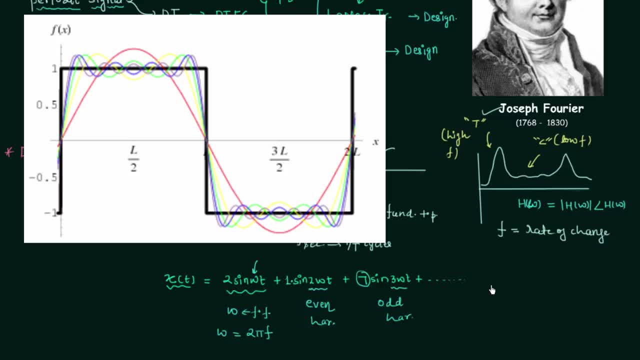 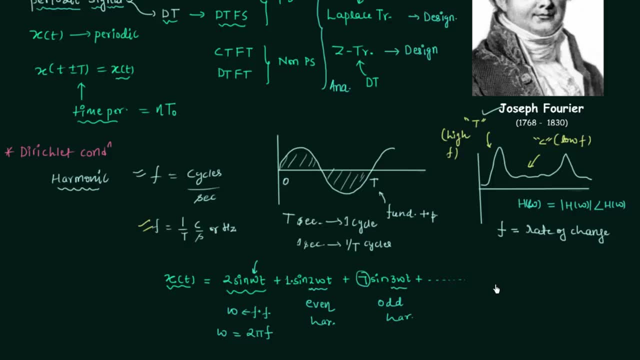 Fourier series. there are other harmonics also, but they are not very dominant, so there is no need to write down all the harmonics. so I hope you now have the clear understanding of the use of Fourier series. now we will understand the last point written in this statement. 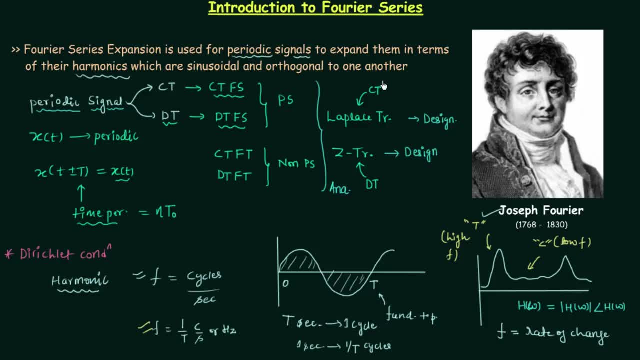 the harmonics are sinusoidal and orthogonal to one another. the harmonics are sinusoidal. this means whenever you have the expansion of the given signal by the help of Fourier series, you will have a dc value plus sine terms plus cosine terms. so we have dc plus sinusoidal terms in the expansion. sometimes 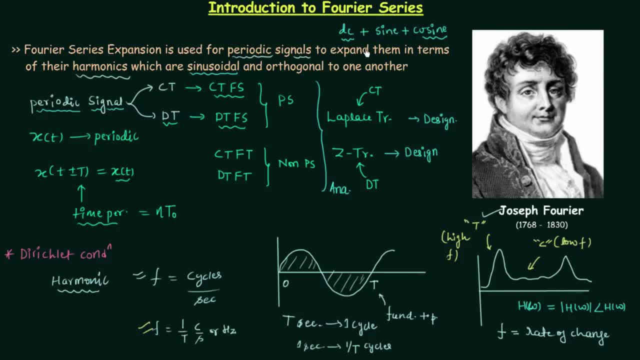 you will have a DC and cosine terms. sometimes you will have sine plus DC. sometimes you will have DC sine and cosine. we will talk more about this in the coming presentations. the next important point is: the harmonics are orthogonal to one another. we already know the meaning of orthogonal: this means perpendicular. 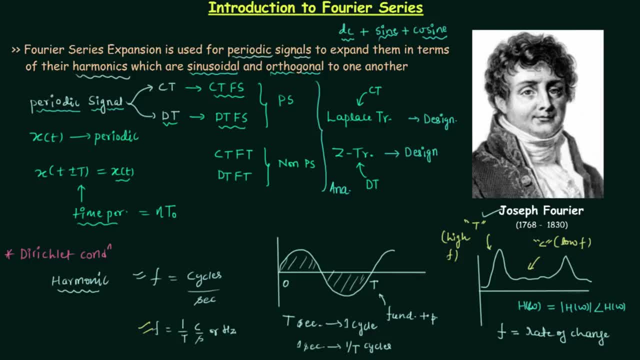 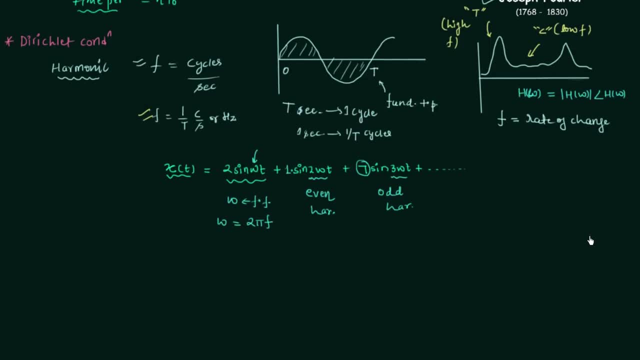 to each other. now let's move to the next point. the next point is: Fourier series is also used to calculate the power and phase content of a particular harmonic present in the expansion, like in this case: you can see the harmonics present in the expansion and we can calculate the phase. 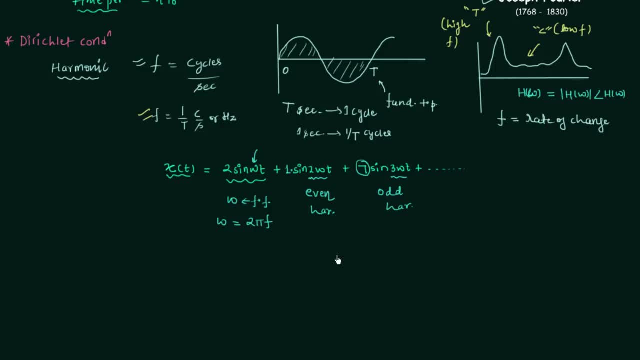 content and the power. easily, therefore, Fourier series is also used to calculate the power and phase content of a particular harmonic present in the expansion. the next point is: power is equally distributed to the harmonics. now we will talk about different types of Fourier series expansion. the first one is known as trigonometric. 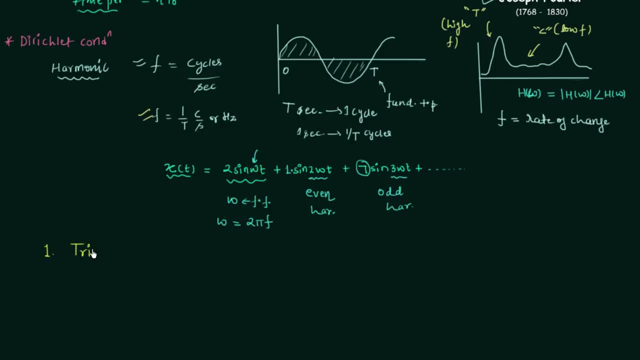 Fourier series expansion. trigonometric Fourier series expansion. the second one is known as complex exponential Fourier series expansion, complex exponential or simply the exponential exponential Fourier series expansion. the third one is known as polar or harmonic Fourier series expansion. polar or harmonic Fourier series expansion for the series expansion our 3. well, first a study, trigonometric. 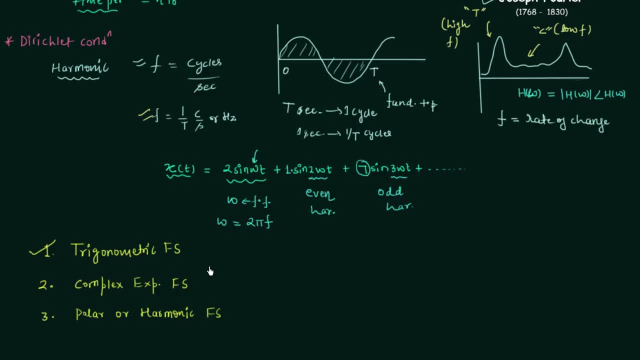 Fourier series expansion. it is important for your college examinations. after this I will explain complex exponential Fourier series expansion following related combinations that is repeated in a parallel Harman Kervei S Tutorial: Fourier series expansion. This is very important and we will focus more on complex exponential 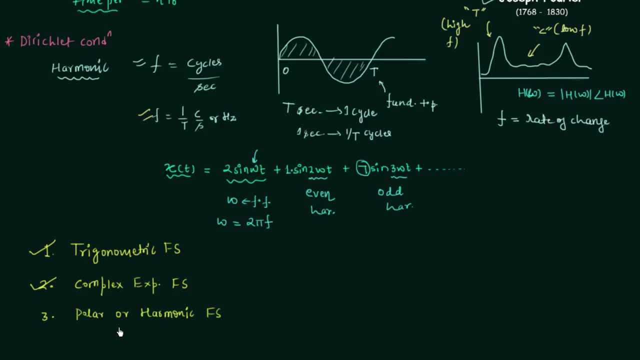 Fourier series- expansion. The third one is polar or harmonic Fourier series. It is not very important And if we have time at the end of this course then maybe I will upload one or two lectures based on polar or harmonic Fourier series. For now, we will focus on 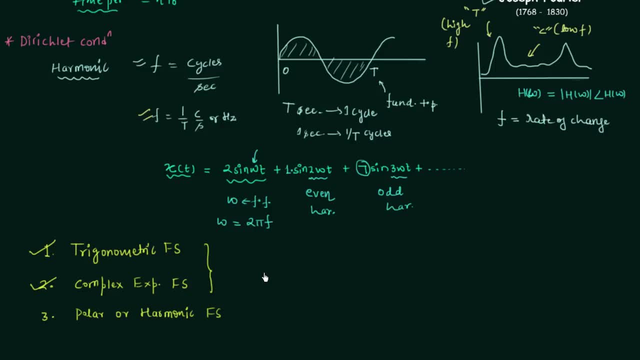 the first two types And in the next lecture, as I already told you, we will start with the conditions for existence of Fourier series, that is, Dirichlet conditions. So this is all for this lecture. If you have any doubt, you may ask in the comment section. This was: